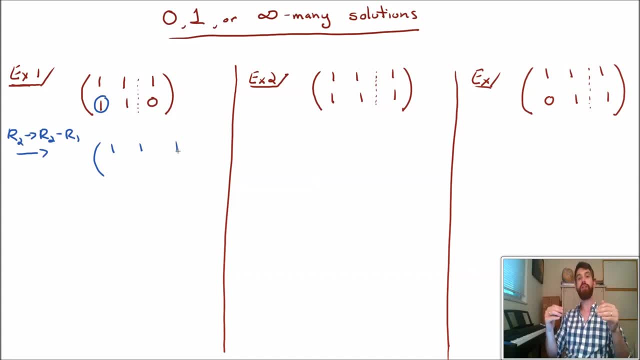 I can just copy and paste the first row, But then if I'm trying to subtract the first row from the second row, I go: 1 minus 1 is 0,, 1 minus 1 is 0, and 0 minus 1 is minus 1.. 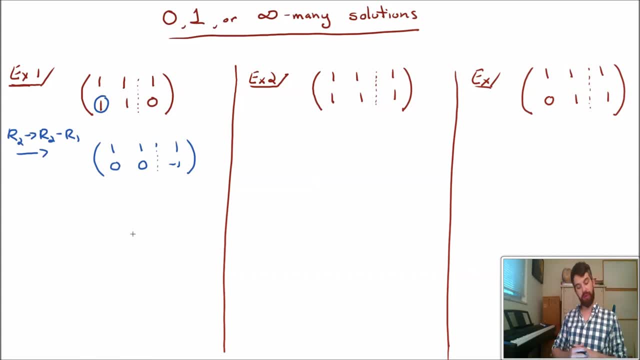 So this is what happens when I try to reduce this particular matrix. However, if I read off the bottom row here, what this tells me is that 0x1 plus 0x2 is equal to minus 1.. In other words, it's telling me that that 0 is equal to minus 1.. 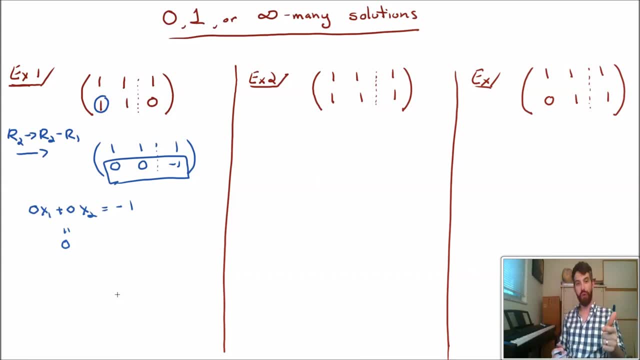 This cannot be. There is no x1 and x2 that has the property that this linear combination of them is going to be equal to minus 1.. So this tells me that I have no solutions, Or another way to write. it is to say that it is inconsistent. 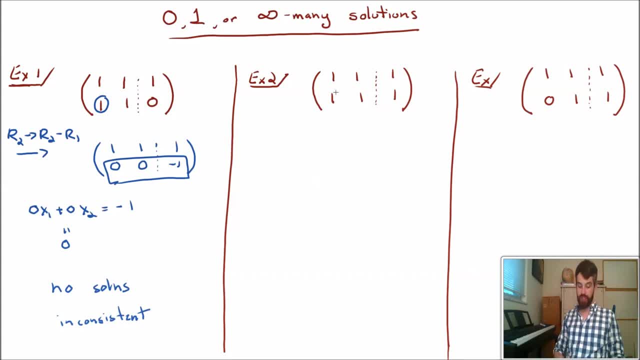 Alright, let's look at the second one. So, same process. I'm going to focus on trying to put a zero in this location And I'm going to do the same thing. I'm going to take my second row and in its place, I'm going to take the second row minus the first row. 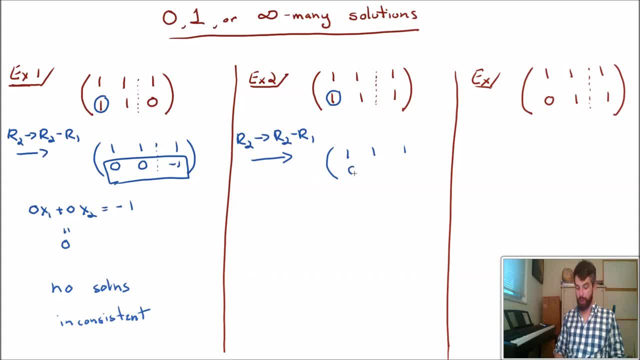 And again, that does not change the first row. But now I go: 1 minus 1 is 0,, 1 minus 1 is 0, and 1 minus 1, one last time is one more zero. Now there's something sort of interesting to note here. 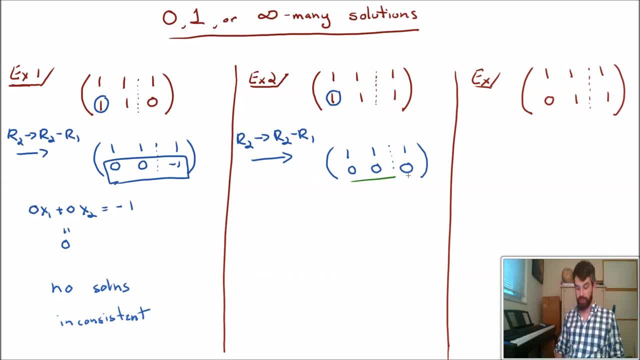 If I look at this bottom equation in this scenario, right. so if I look at the bottom row, this is a totally pointless row. It just tells me that 0x1 plus 0x2 is just equal to 0.. Well, duh, It doesn't matter. 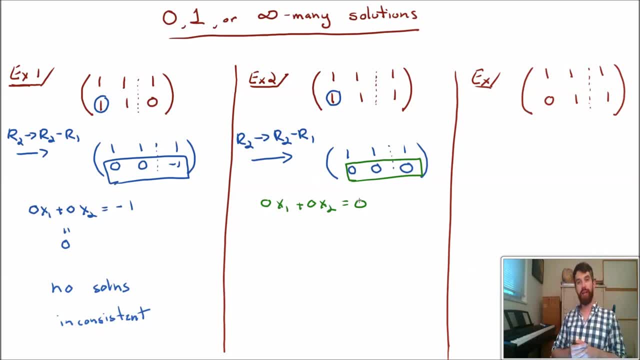 I'm getting. I'm not getting any new information, Or another way to put it on. it is that I am not putting any constraint on the variables x1 or x2.. In a sense, I have a little bit of freedom here. 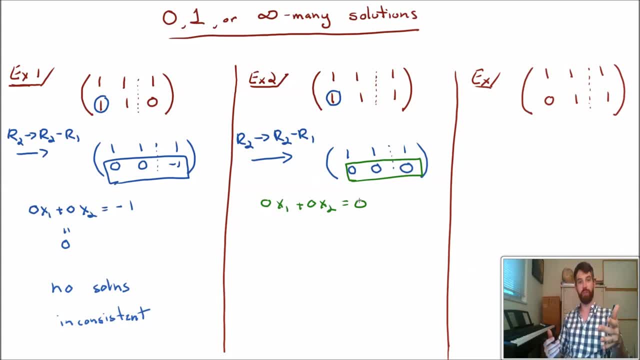 That normally I had two different equations that would constrain my variables, But now I only have one equation that's constraining them, the first of them. So what I'm going to do is this: I'm going to let x2, it could have been x1, but I'm going to let x2.. 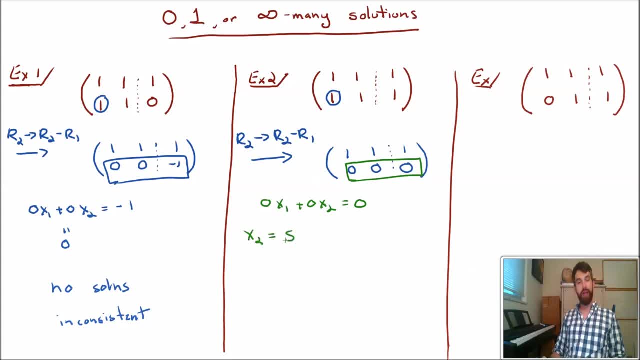 And I'm going to let x2 equal to s, And when I do this, I'm thinking of s as just some arbitrary free parameter. So this s is a free parameter, It could be anything. And then what I'm going to do is I'm going to figure out what x1 is in terms of this parameter. 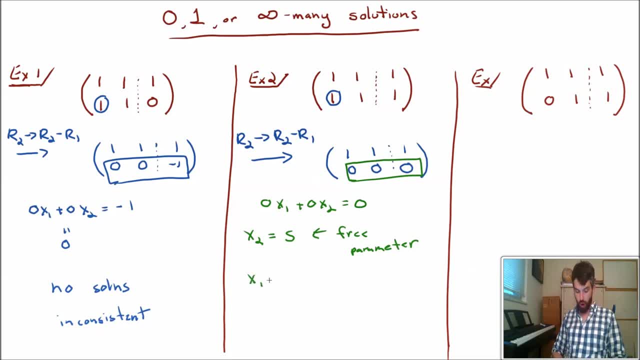 which could be anything. So I'm going to say, therefore, from the first row: x1 plus x2 is equal to 1.. So, in other words, x1 plus that value that I'm substituting it, in, which is s, is equal to 1.. 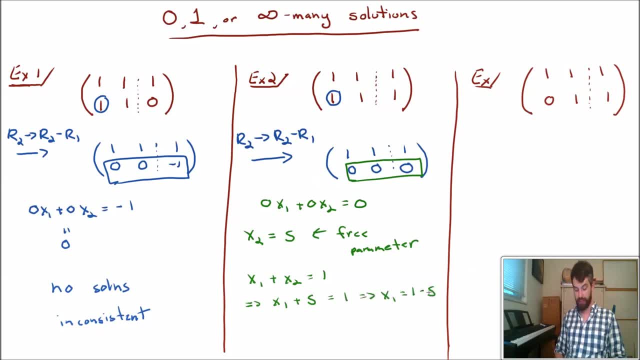 Or in other words, x1 is equal to 1 minus s. So if I take those things together, what you'll notice is that there are infinitely many possible solutions. Infinitely, Infinitely many solutions. Why, Well, choose any number s you might like. How about 100?? 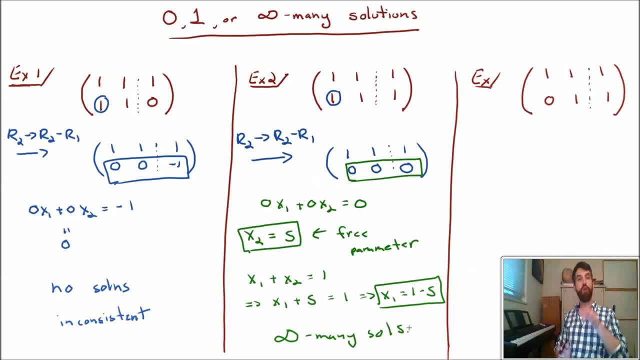 Then that can be my x2, and my x1 is going to be 1 minus 100, or minus 99 in this case. So for any value s that you can get, we get a pair- x1, x2,, which is going to solve this system. 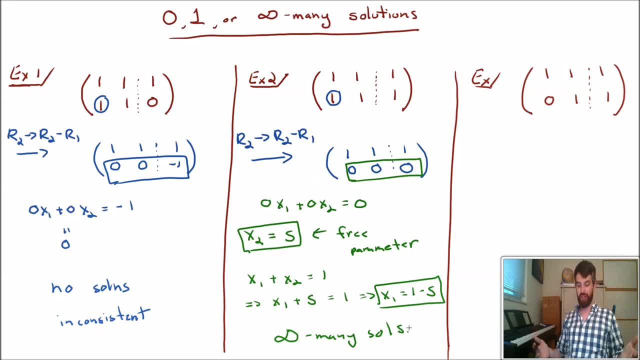 of linear equations, And so the idea is, effectively, when you have these zero rows that don't put any constraint, then you get some freedom and you just make one of these variables, in this case the x2, a so-called free variable or a free parameter. 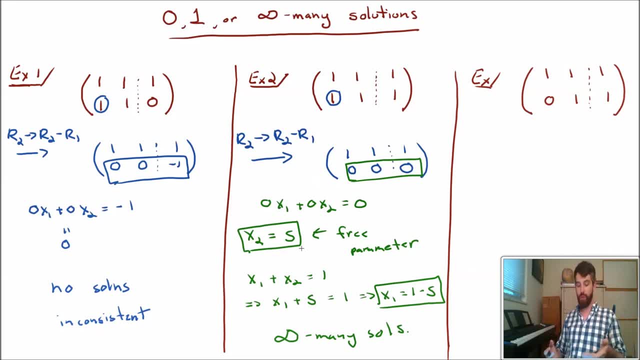 It could just be any arbitrary symbol s, And then you figure out what the other variables can be in terms of that free parameter s, And then in this final one, it's already in that form that I want to have, where I've got a leading one here and then a zero beneath it and then another. 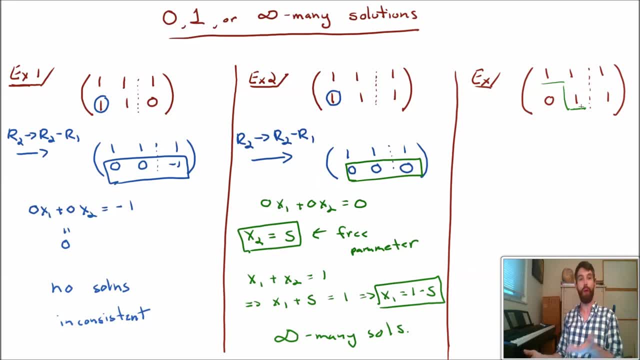 leading one here. I actually don't need to do anything. It's already in its ideal situation And I can just read off. So if I look down at the second equation, I get: x2 is equal to 1, so that's one answer. And then for the first equation, I get: 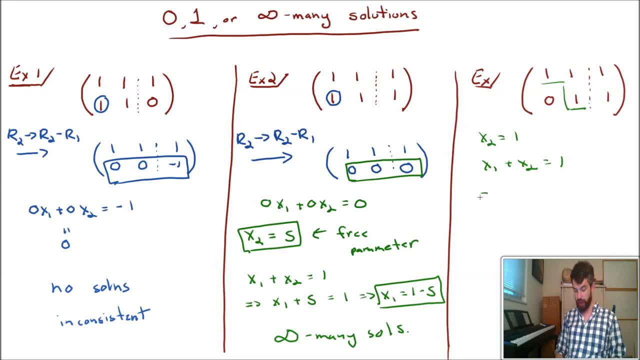 x1 plus x2 is equal to 1, so, in other words, x1 plus 1 is equal to 1, or, in other words, x1 is equal to 0.. So, in other words, I'm going to just get one solution, a unique solution.